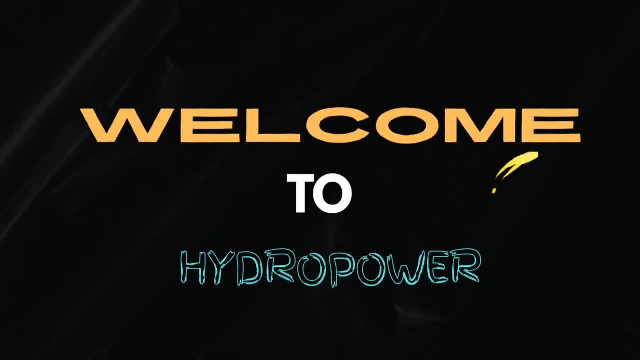 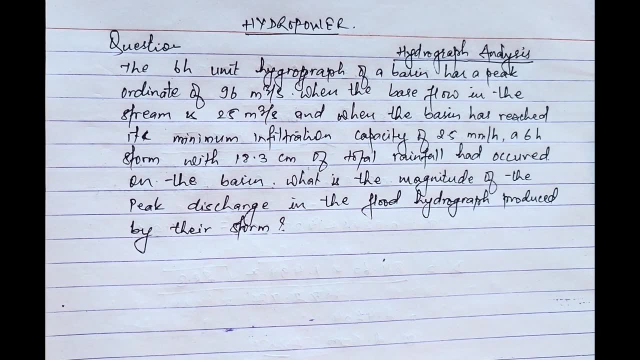 Hello everyone, welcome to hydropower Today. in this video we will solve one numerical problem related to hydrograph analysis. So the given question is: the six hour unit hydrograph of a basin has a peak ordinate of 96 meter cube per second, when the basin flow in the stream is 25. 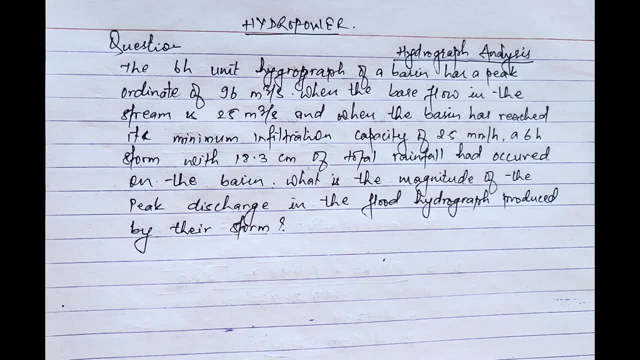 meter cube per second and when the basin has reached its minimum infiltration capacity of 2.5 mm per hour, a six hour storm with 18.3 cm of total rainfall had occurred on the basin. What is the magnitude of the peak discharge in the flood hydrograph produced by the storm? This is the 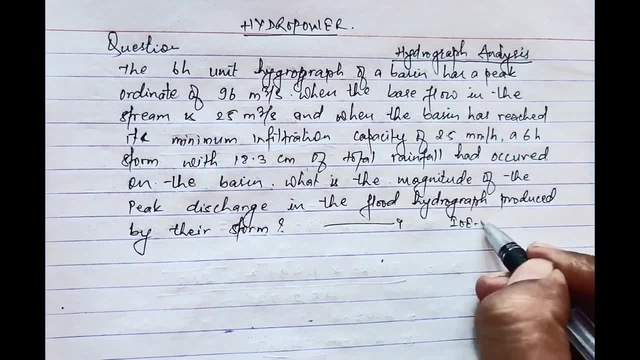 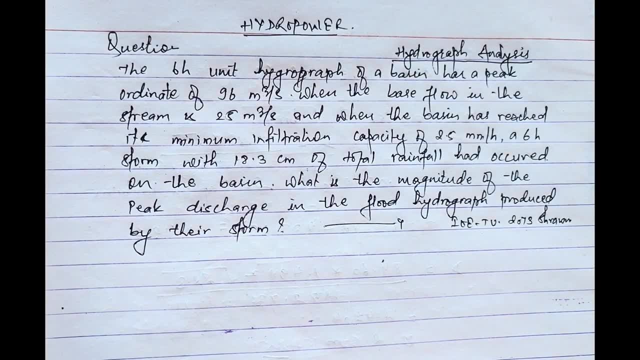 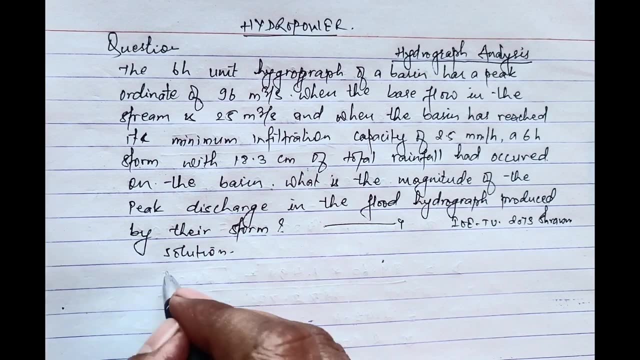 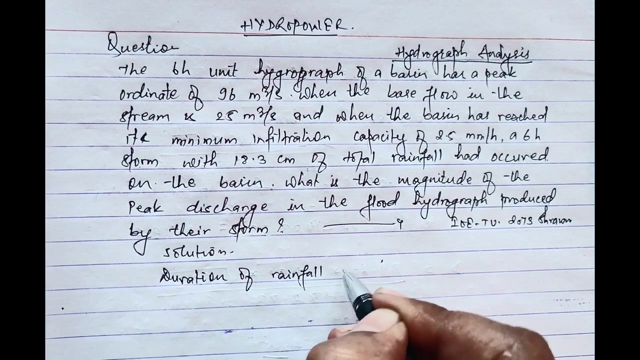 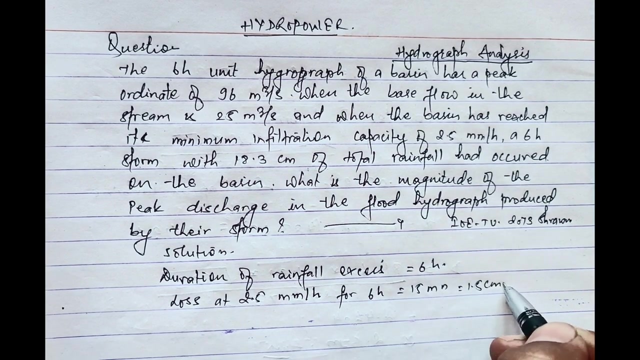 world question of I O E T U on 2070. 3.. So let's start this question with the solution Here. the duration of rainfall access equals six hour loss at 2.5 mm per hour. for six hour equals 15 mm. 6 into 2.5 goes to 15 mm, that is 1.5 cm. so the total rainfall 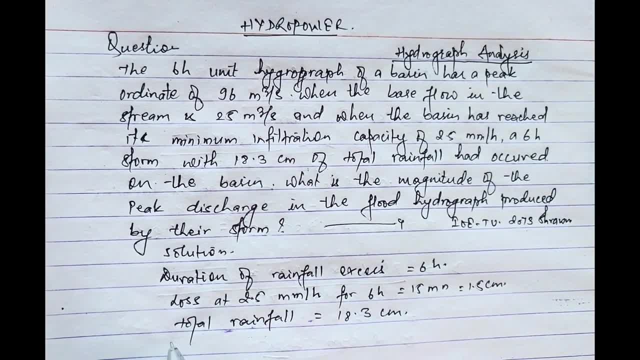 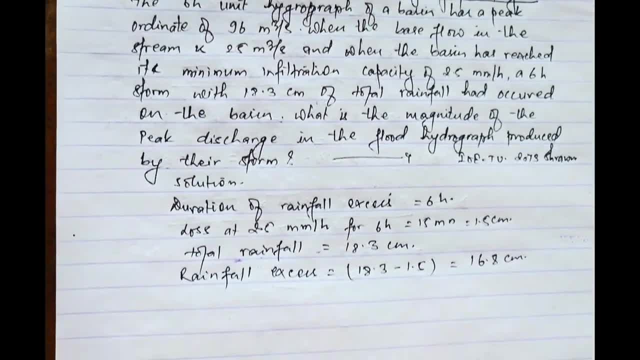 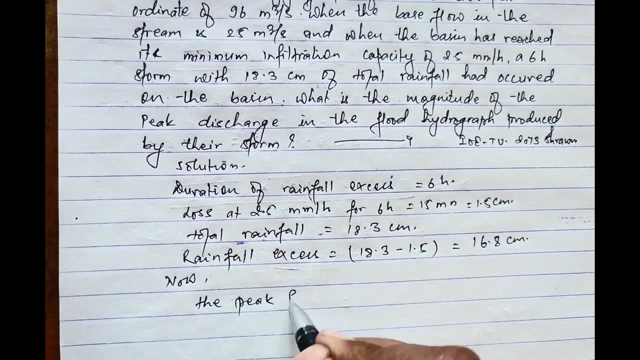 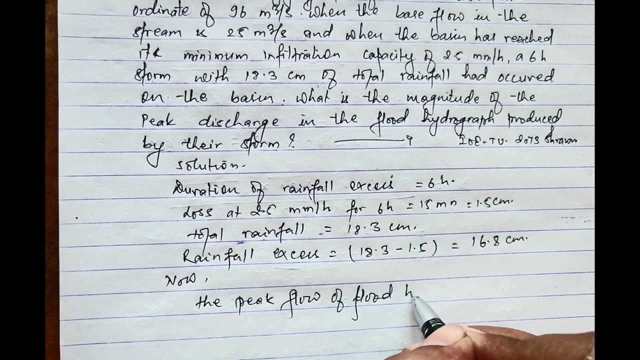 6.5., 6.5., 6.5., 6.5., 6.5., 6.5.. Now the peak flow Flow of Flood hydrograph Equals 96. Meters per Second.